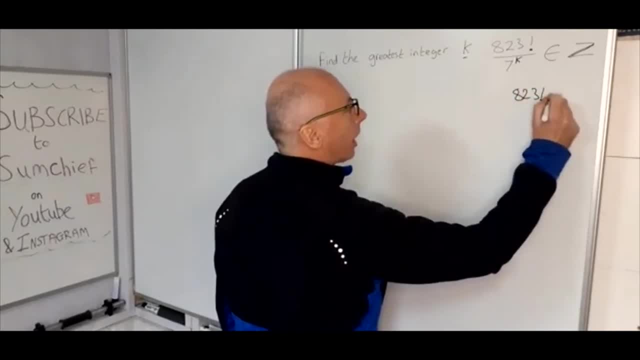 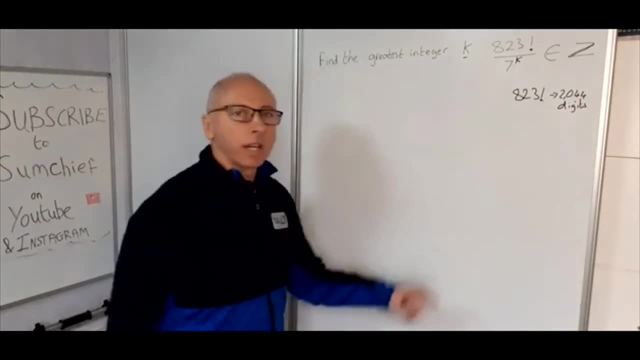 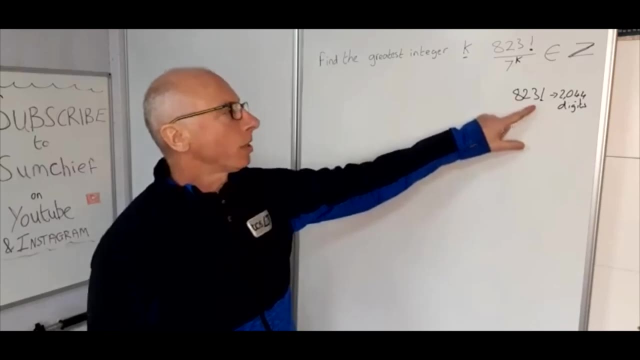 has 2044 digits. Now, if you follow the link below, I'm going to show you how to calculate how many digits there is and how many trading zeros this has. So let's go ahead and do that. There's going to be so many zeros at the end of that as well, So I'll follow the link. 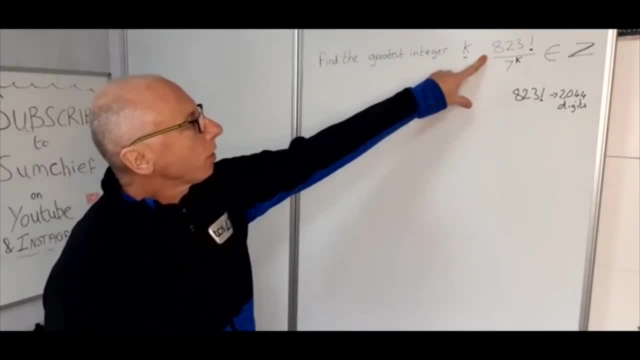 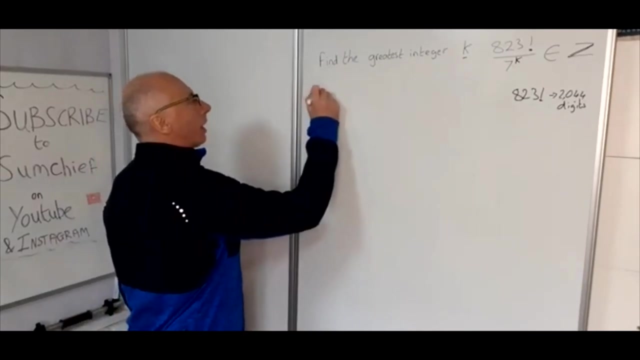 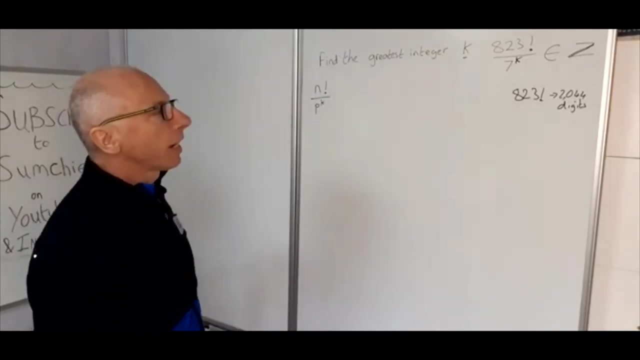 and I'll show you that. So back onto this question. 823 factorial divided by 7 to the power of k. We also see that 7 is a prime number. That's also really helpful So we can use a particular formula. So we've got n factorial divided by a prime number to the 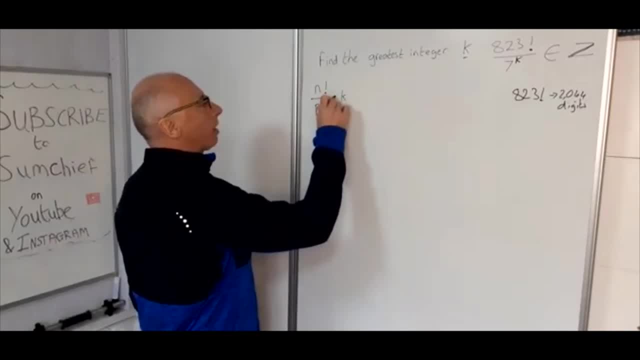 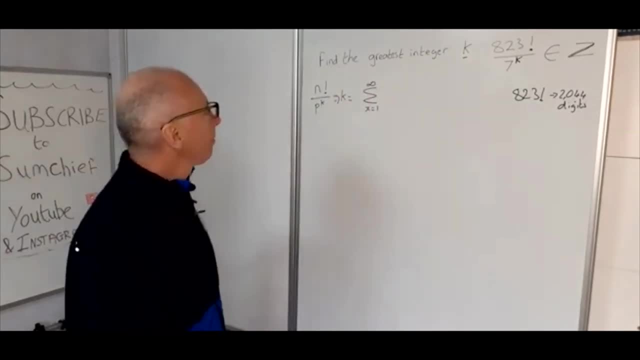 power of k. So what we do is we have k equals the sum of x, equals 1 to infinity, And we use something called. we can use the floor function or we can use the greatest integer function. This time I'm going to use the greatest integer function. It's going to give us the same result. 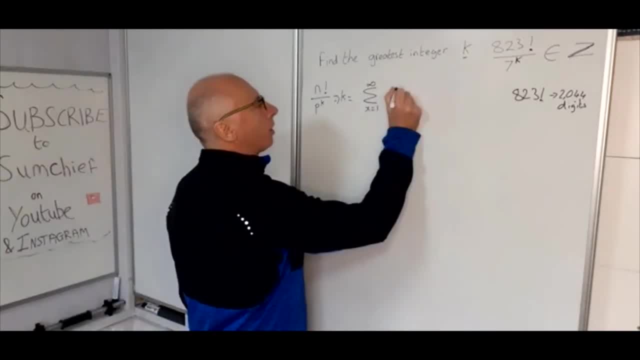 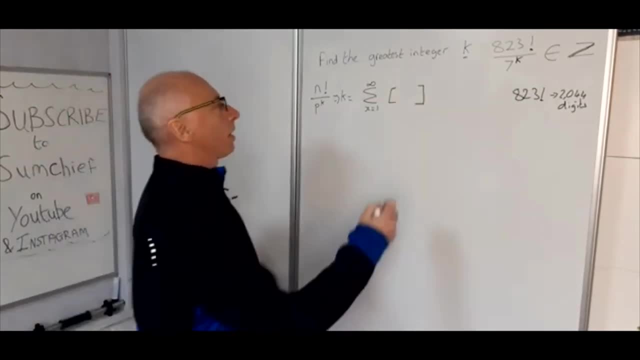 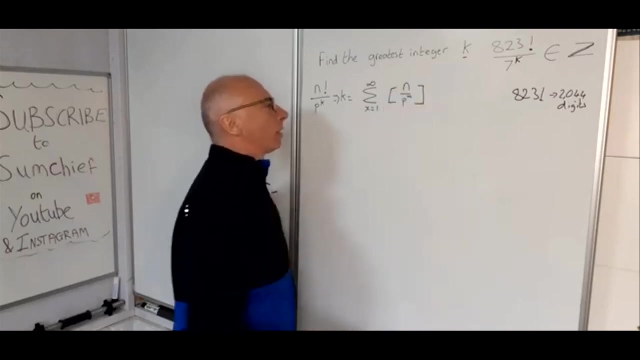 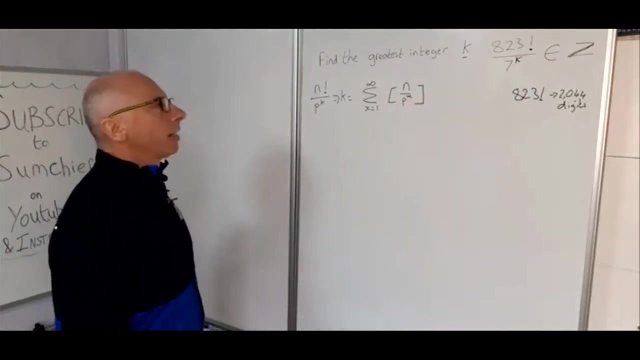 but it's just different notation. So greatest integer function is basically two square brackets and then a number inside, And then we're going to have n divided by p to the x. So you can see what's going to happen here. We're just going to sum them all up over p to the x's. Okay, So here? 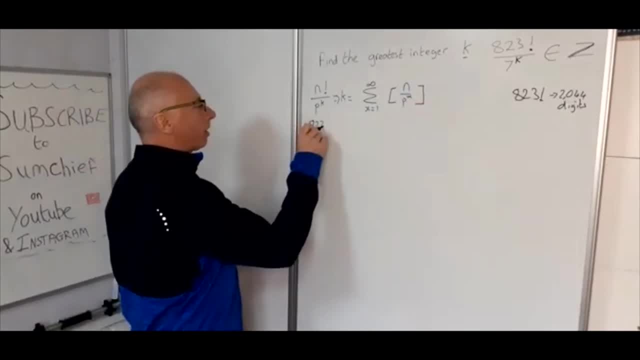 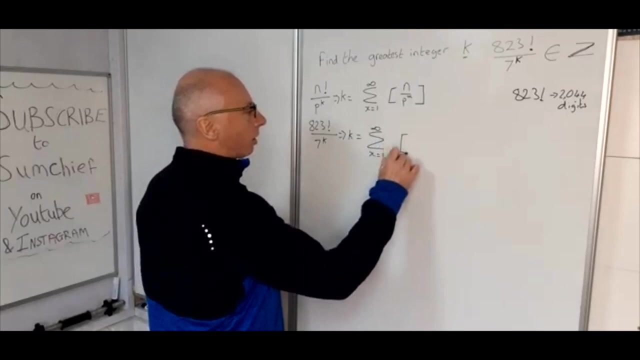 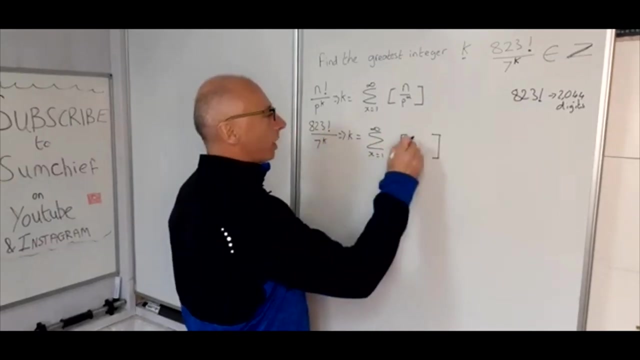 we've got 823 factorial- I'm going to write that down again here- Divided by 7 to the power of k. So we want k. So k equals x, equals 1 to infinity, Greatest integer function. And 823 is our n and our p is 7,. 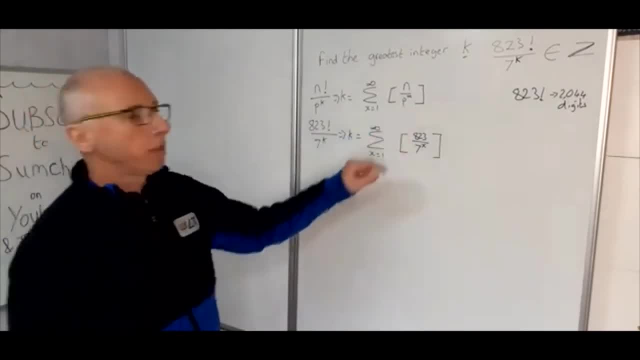 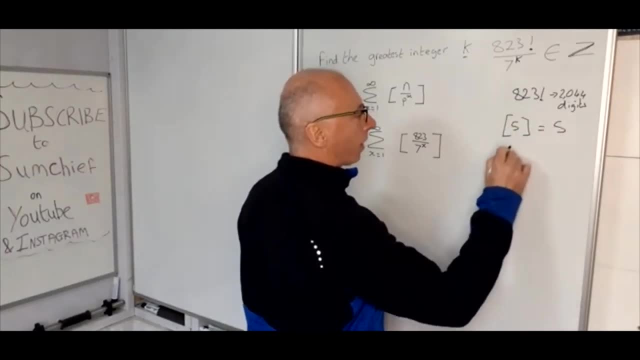 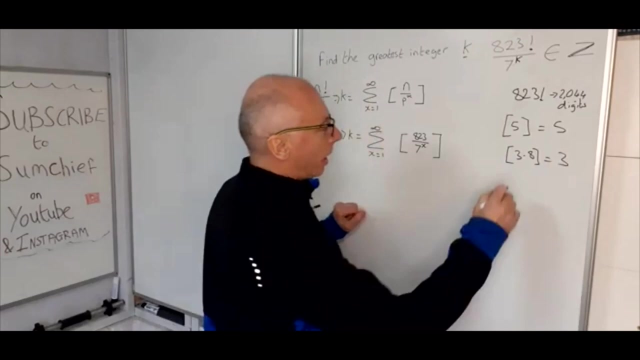 that's to the power of x. And just to confirm this greatest integer function, if we have greatest integer 5, that equals 5.. So we've got: k is greater than or equal to 823.. And we're going to equals 5. the greatest integer, 3.8, that equals 3. and then the greatest integer 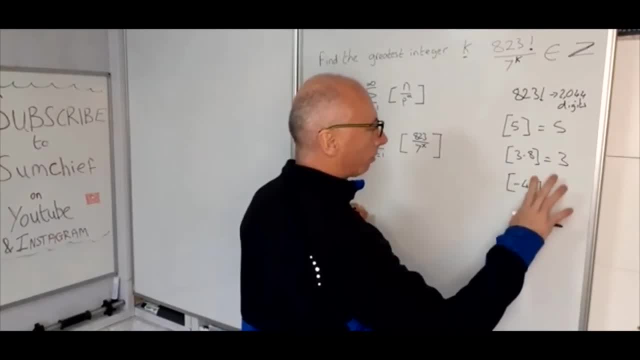 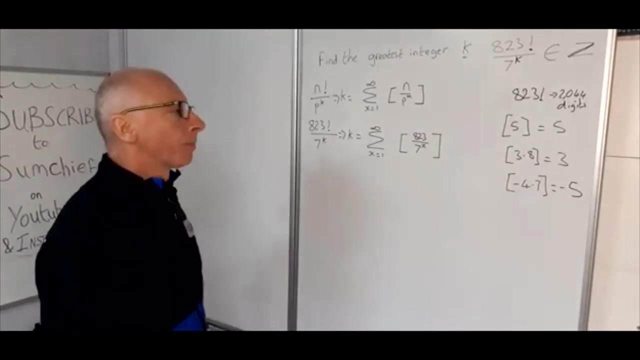 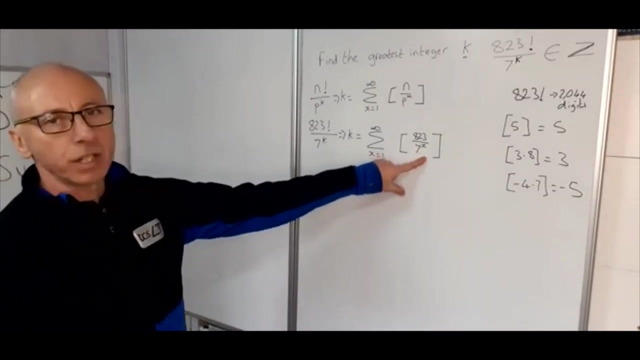 minus 4.7. 4.7 that equals minus 5, but we're moving down from minus 4.7, we're moving to the lower number. okay, back onto this 823 divided by 7, to the x and the greatest integer of that. so with a summation formula, it's just simple: we just plug in all the different values. 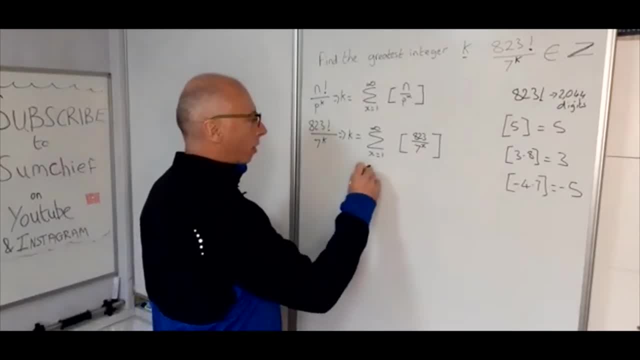 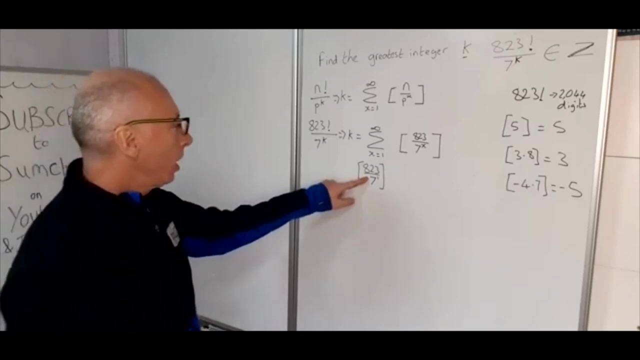 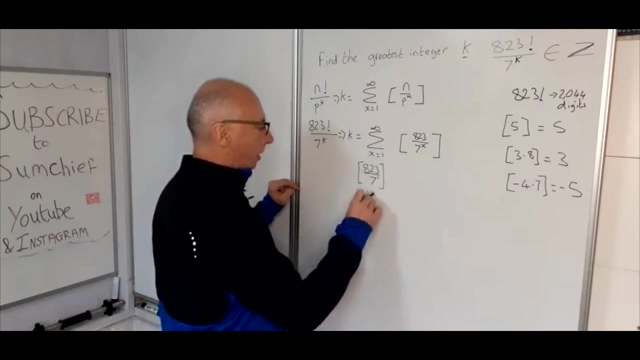 of x and see where that takes us. so for the first one. so for x equals 1, we've got 823 divided by 7 to the power of 1, taking the greatest integer of that. well, how many 7 are there in 823? Well, 7 into 840 will be 120. so we got 117. so that would be our floor function. 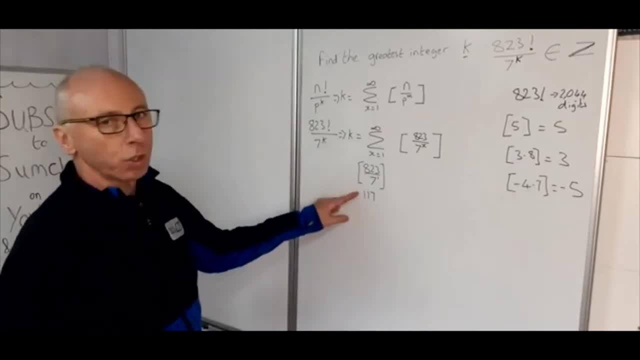 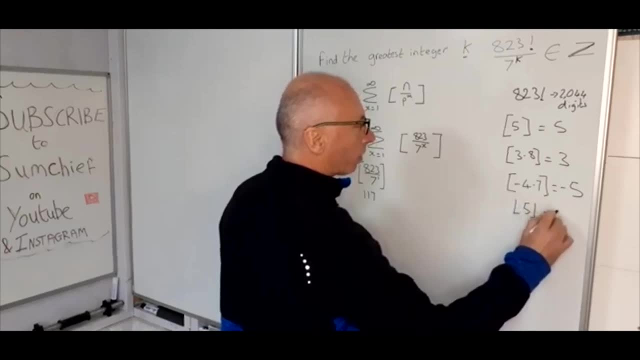 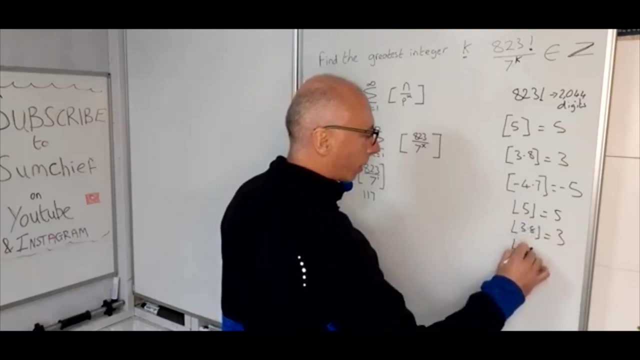 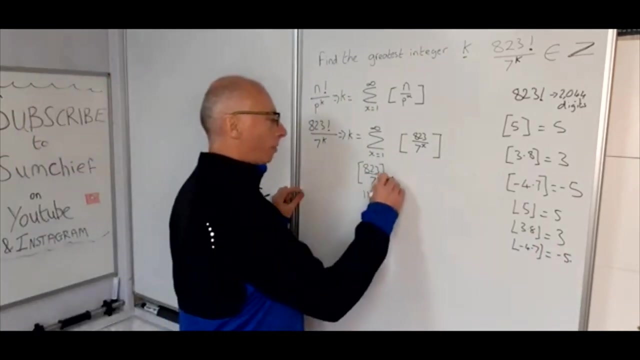 value, sorry, our greatest integer value. here you could also use the floor function, like I just mentioned. so same with these: the floor function of 5 equals 5, the floor function of 3.8 equals 3 and the floor function of minus 4.7, that equals minus 5, 2.. So that's the first one. Now we move on to x equals 2.. 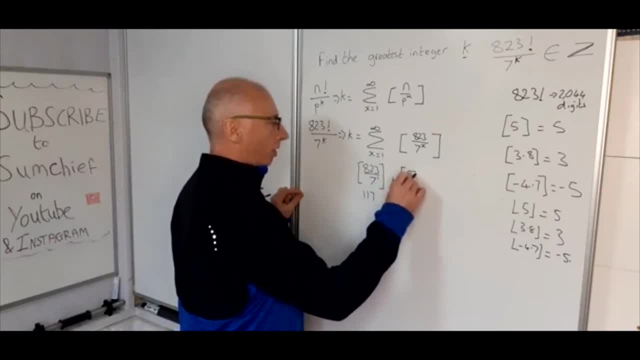 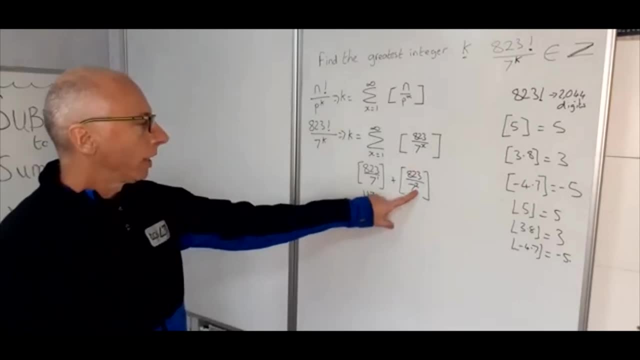 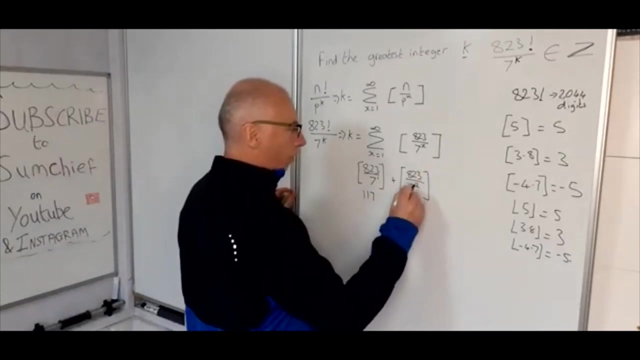 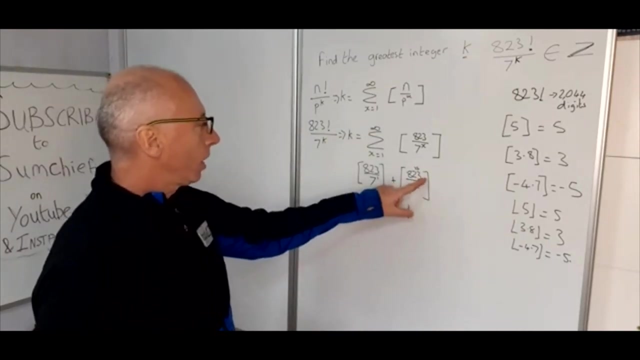 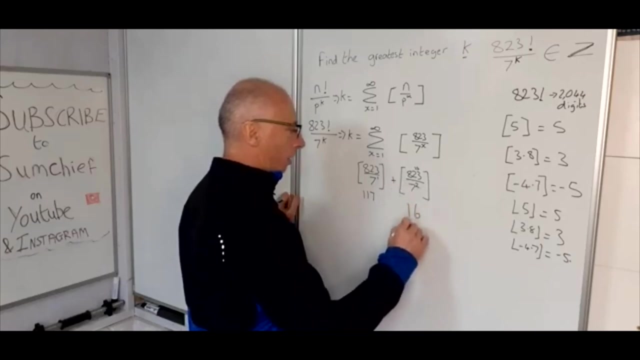 So greatest integer function, 823 divided by 7 squared. Now, 7 squared is 49.. So 49 into 823, or we got 1 with 33 left over, 49s into 333.. That's going to be 16 altogether, isn't it? 16 times 49.. Let's just work that out: 49 times 16. 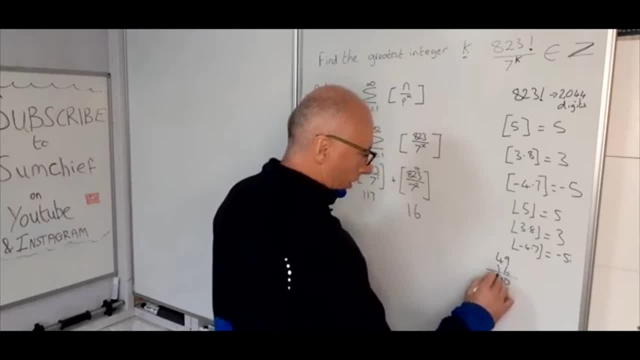 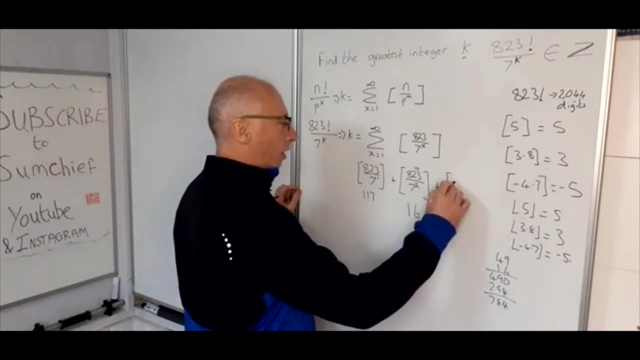 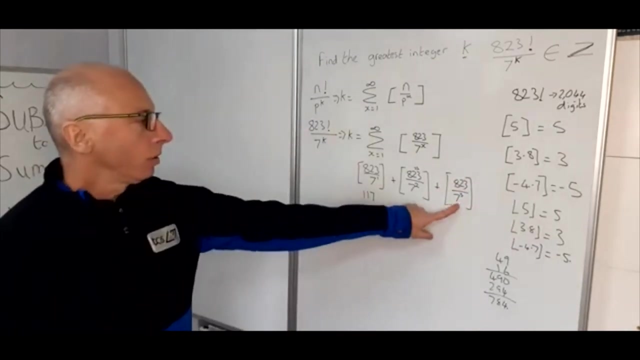 490, 65, 300, 294. that gives us 7, 8, 4.. So yeah, that's perfect for us. So that's 16.. Now on to the next one: 823, 7 cubed. So 7 cubed is 49 times 7, which is 343..